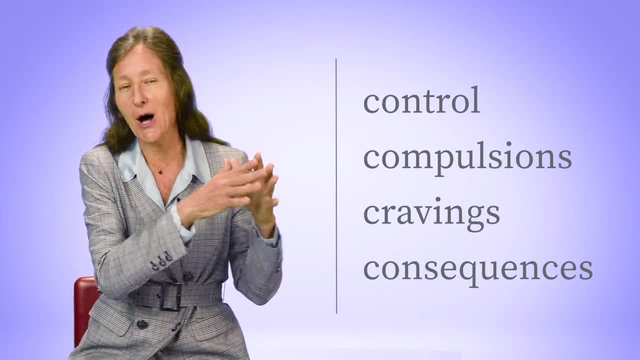 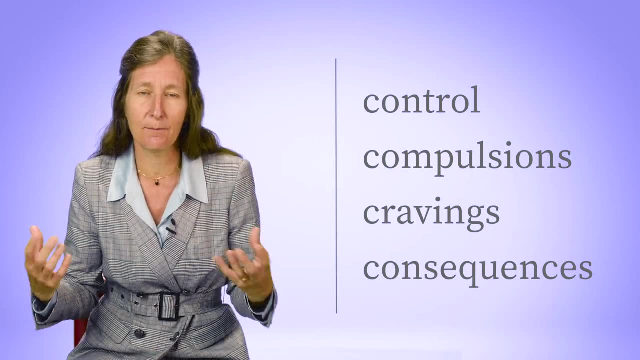 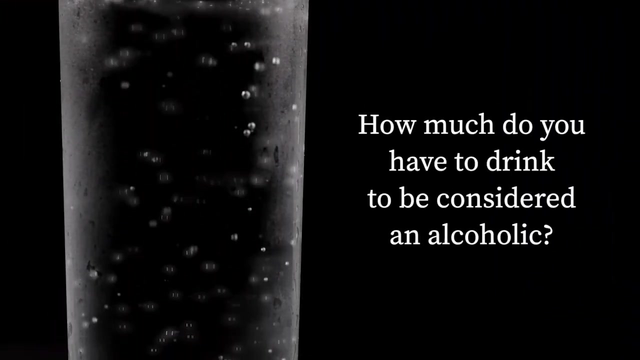 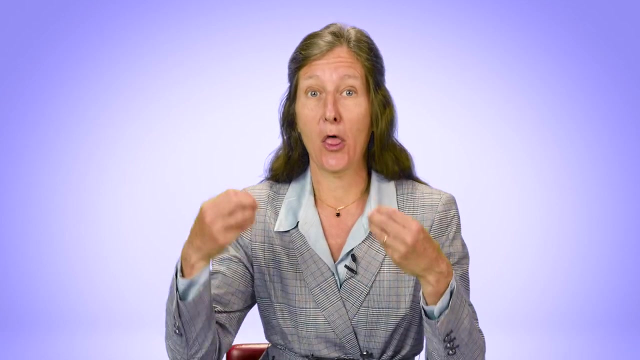 characterized by tolerance and withdrawal. those four C's alone, which represent the complex biopsychosocial disease of addiction, can constitute meeting threshold criteria in and of themselves. How much do you have to drink to be considered an alcoholic? Quantity and frequency of alcohol consumption really matter The more you. 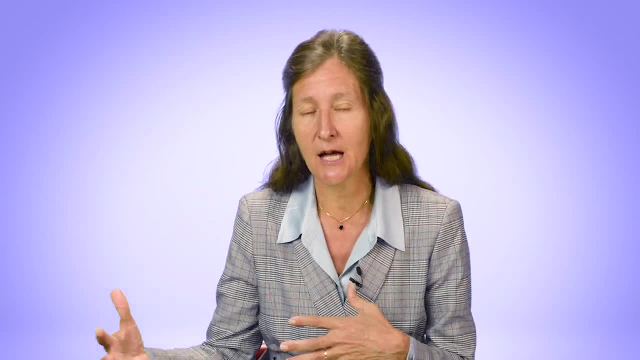 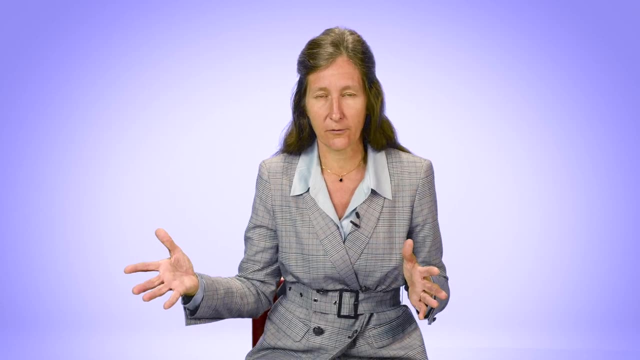 drink, and the more often you drink, the more likely you are to meet the diagnostic criteria for addiction. But the diagnosis itself is not dependent on quantity and frequency. It's dependent on those four C's we talked about. How much do you drink? 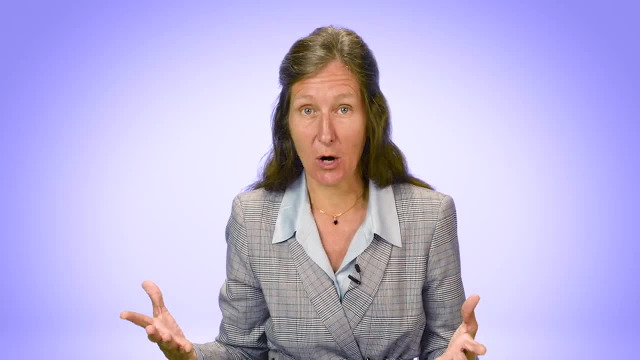 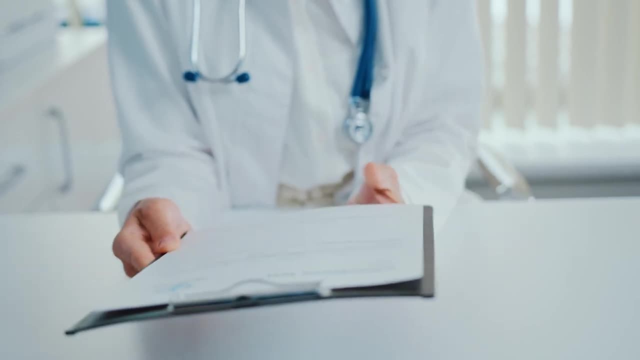 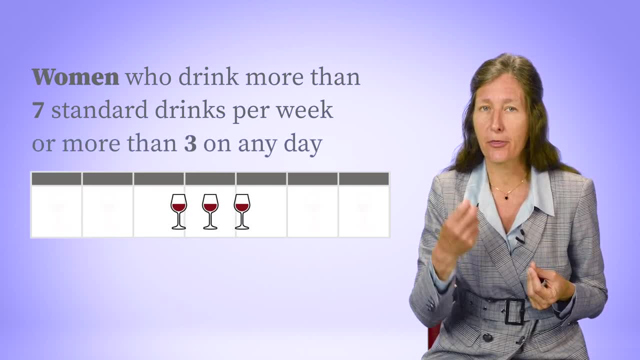 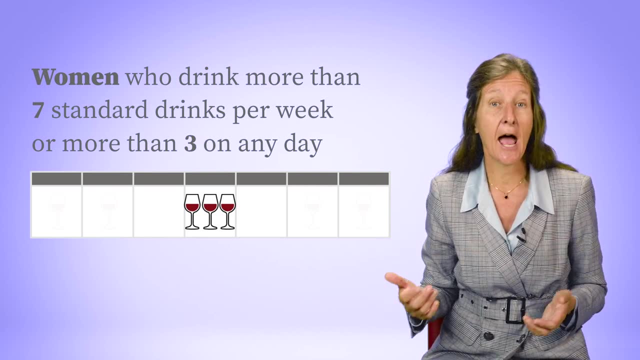 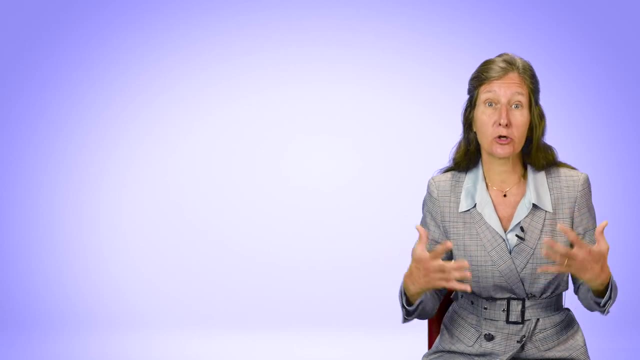 So the five to 7 standard drinks per week, or more than three on any given day, are at greatly increased risk for all cause, morbidity and mortality, And are also more likely to meet criteria for addiction to alcohol. For men, those numbers are higher For men who drink more than 14 standard drinks. 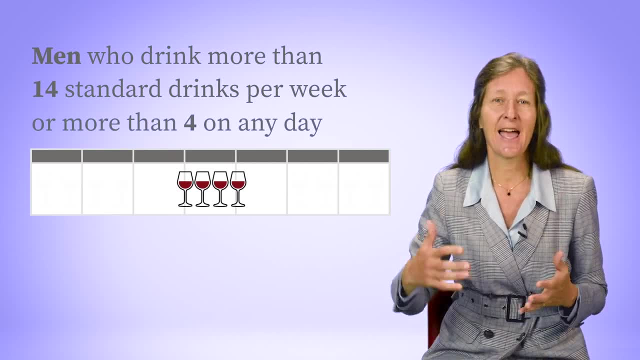 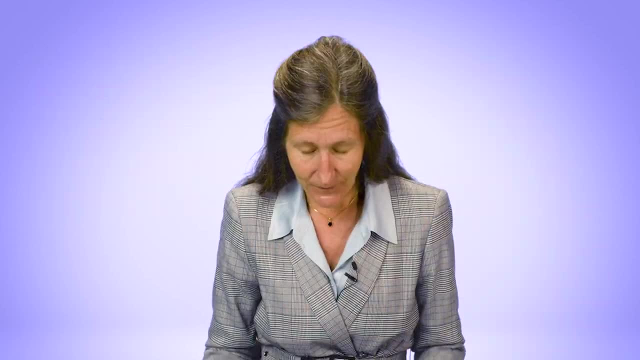 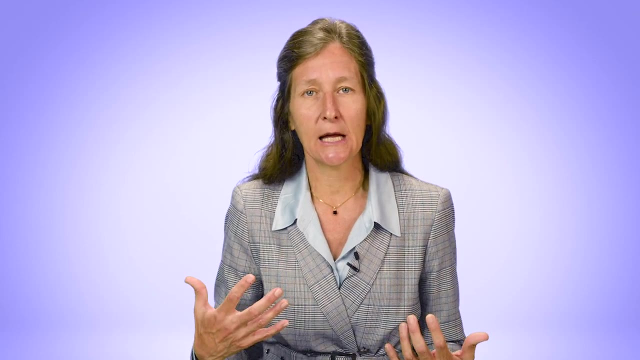 per week or more than four drinks on any given day. their risk of all cause, morbidity and mortalitygoes way up in their daily consumption, including the risk of addiction. why are there differences? there's something about female metabolism that makes drinking in very large amounts. 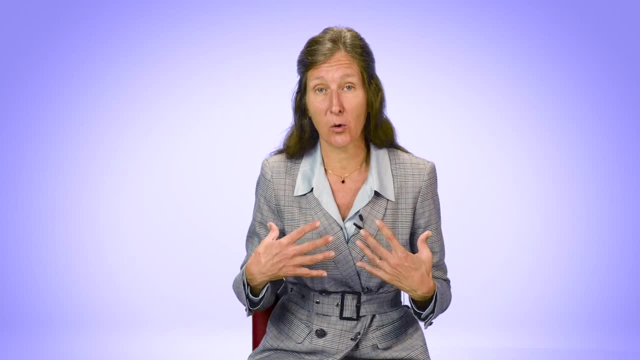 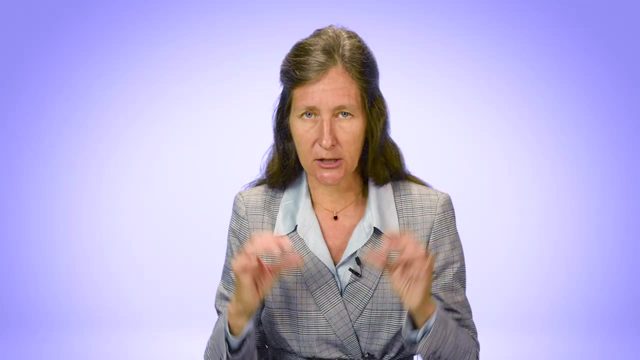 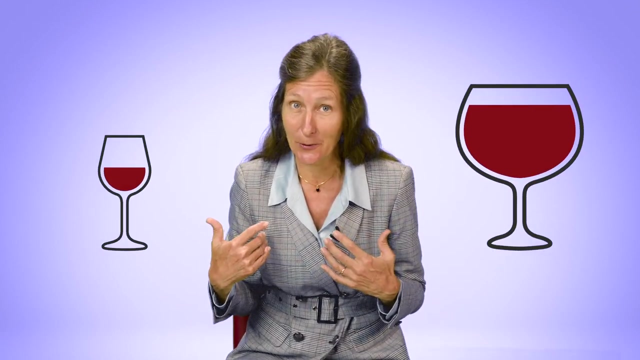 potentially riskier and more dangerous for the organs than in men. what's a standard drink? okay, so let's talk for a second about what a standard drink is, because that's really important, right? so your, your glass of wine and my glass of wine may look really, really different. we define one standard drink as one 12. 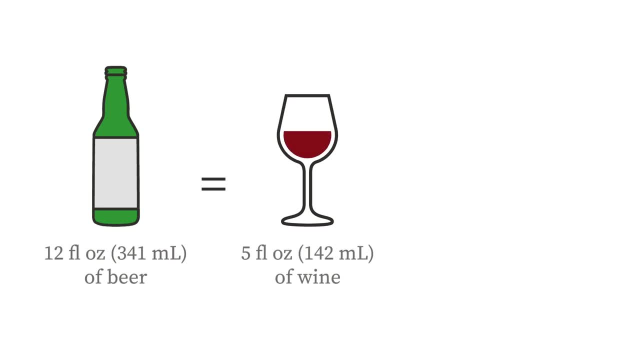 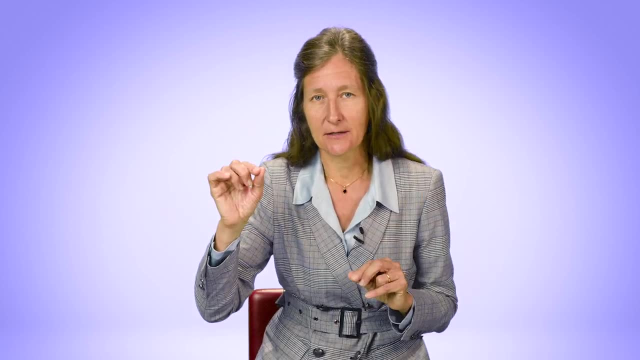 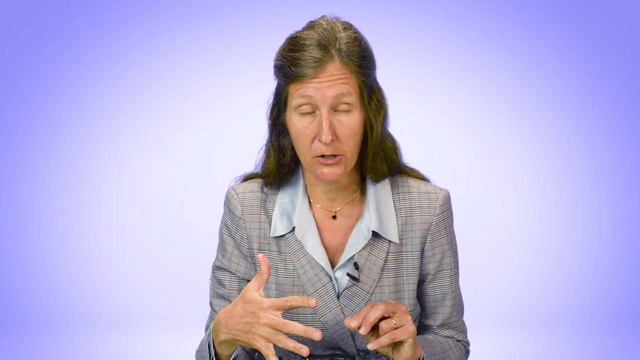 ounce bottle of beer, one five ounce glass of wine, or about one to one and a half ounces of hard liquor. okay, so I've given you the limits. a couple caveats there. once men hit the age of 65, their drinking standards come down to where women are. also, these limits are the upper limits, in fact the healthiest. 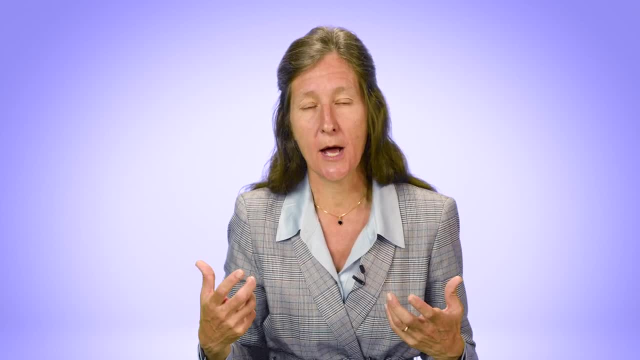 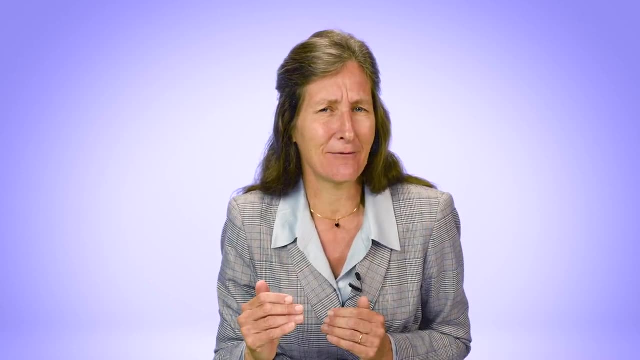 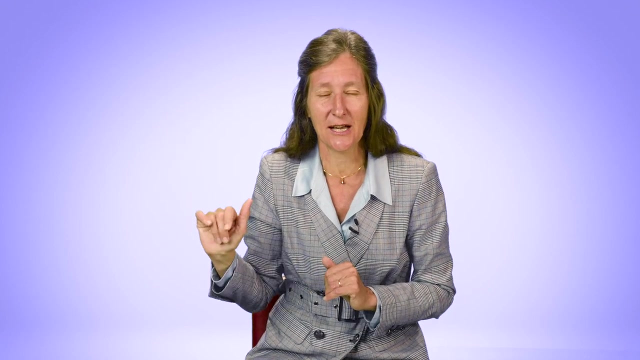 people in the world only have one standard drink in the world, and that's one to two standard drinks per week. that's really really important, okay. so if you're brushing up against that seven per week if you're a woman, or that 14 per week if you're a man, you're really in a much, much higher risk category. if 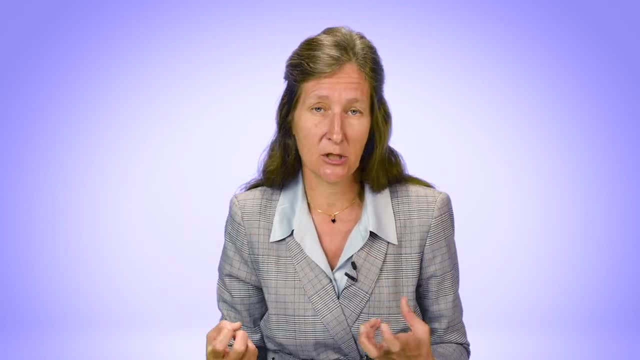 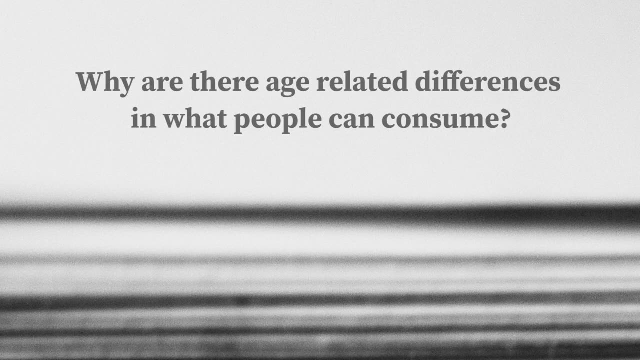 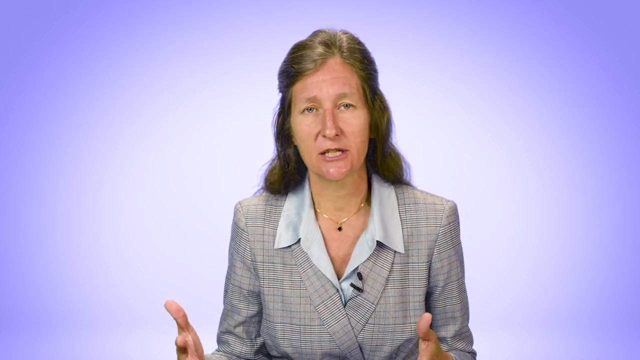 you really want to be super healthy, try to keep your alcohol consumption down to one to two standard drinks per week. why are there age-related differences in what people can consume? we don't really know why, but it looks like as we age, we just simply metabolize alcohol. 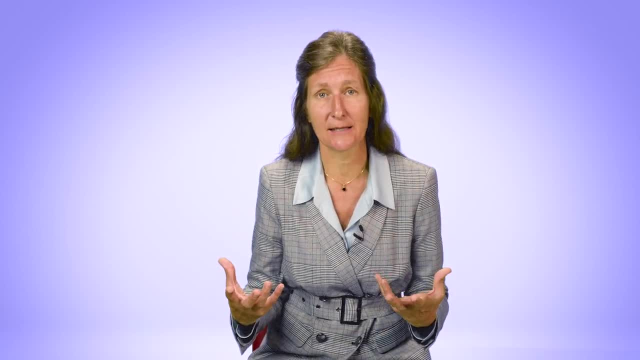 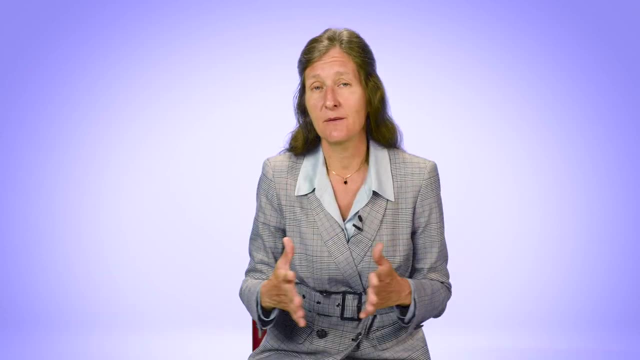 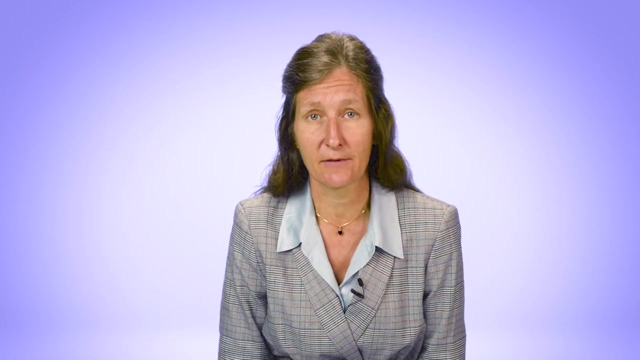 differently and can therefore tolerate less alcohol, which is why the amounts for men decrease at age 65. for women, they stay the same, but in fact it may be that we just don't have enough data, and if we were to look more closely at that, we would need to bring those numbers down for women over 65 as well. does 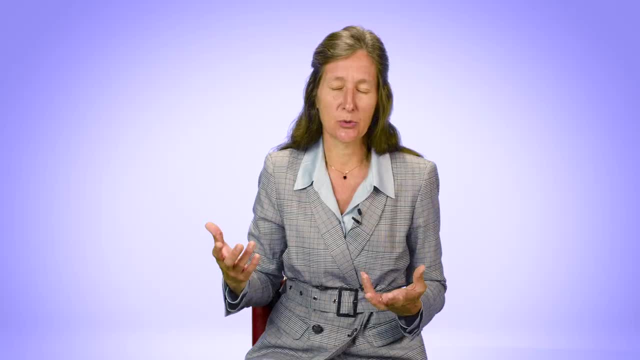 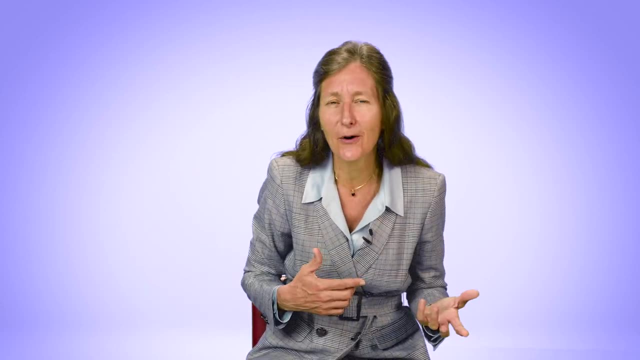 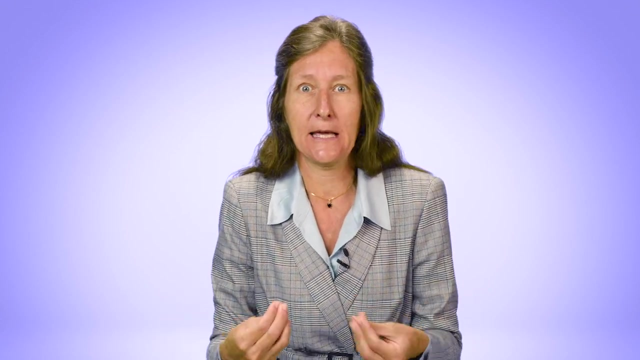 drinking alcohol have any health benefits? patients will say: well, isn't drinking red wine good for me? I mean it has like resveratrol, which is going to help me live forever. and the truth of the matter is that there's no real evidence to support this idea that alcohol in and of itself is healthy. the 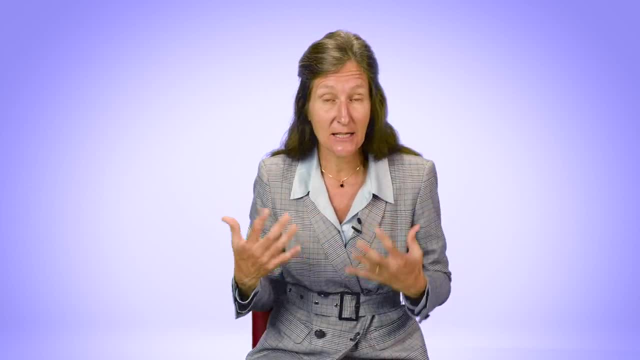 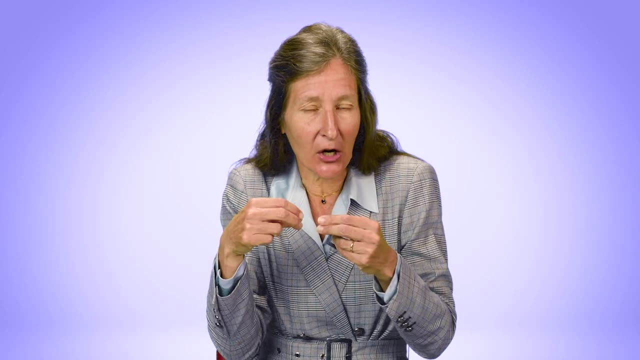 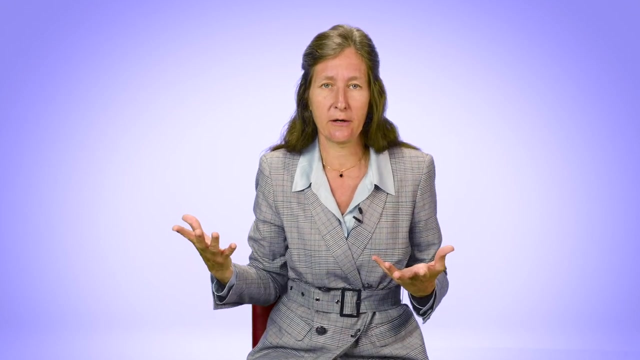 reason that we have that notion is because, in fact, it is true that the healthiest people have no more than one to two standard drinks per week, and they're even healthier than people who drink not at all. so how can that be? again, one putative conclusion from those data is that alcohol is healthy, but in fact, 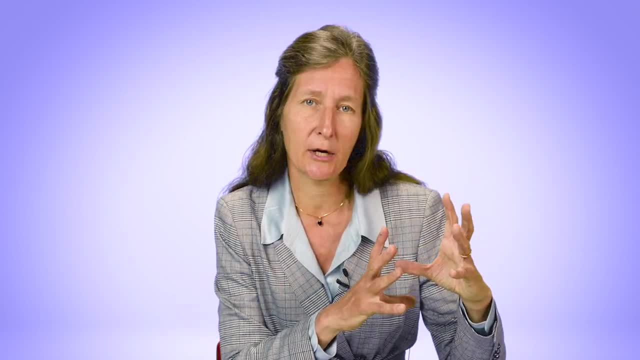 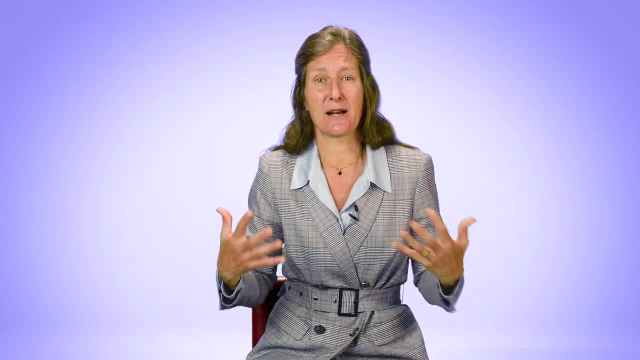 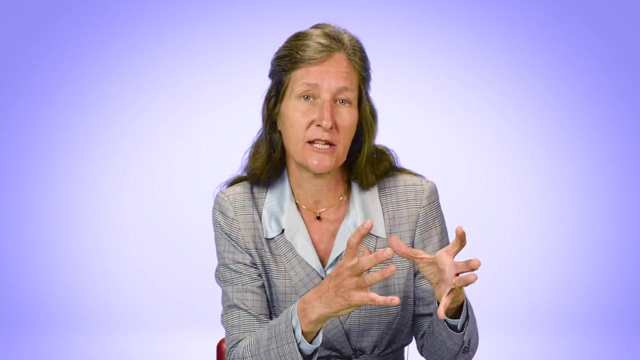 what's really happened is that group of people who don't drink includes a group that we call sick quitters, and those are individuals who have had to stop drinking because they drank so much that it caused liver damage, pancreatic damage, heart damage, brain damage, and they change the overall risk category of